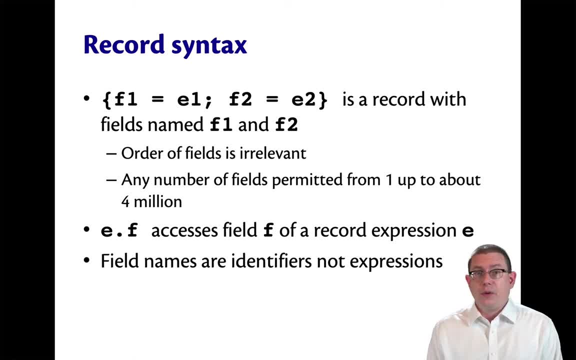 And OCaml will not distinguish one record from another based on the order of the fields. You can have any number of fields you want inside of a record, from one up to somewhere around four million. Honestly, you would never have a record that big really. 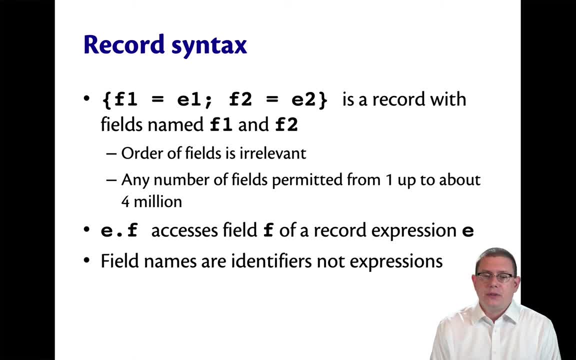 You might have three, four, five, even eight fields. We write dot to access a field from a record, So E dot F accesses the field named F of a record expression E. It's important to bear in mind that F here is a field name and it must be an identifier syntactically. 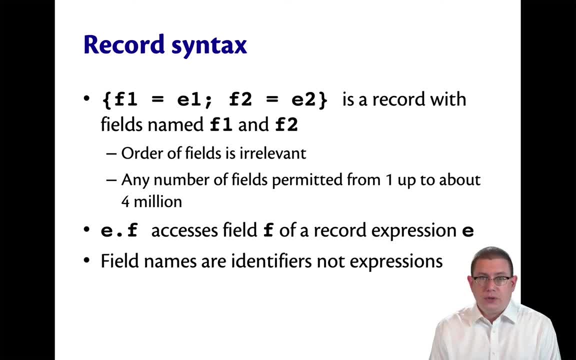 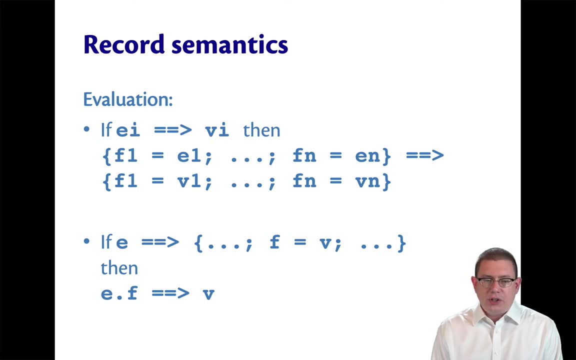 It cannot be an expression that you compute. If the latter is what you want, then really what you are thinking of is a dictionary, And we will come to dictionaries later. How do you evaluate records? It takes a lot of notation and words and math here to write down what's really a pretty simple concept, honestly. 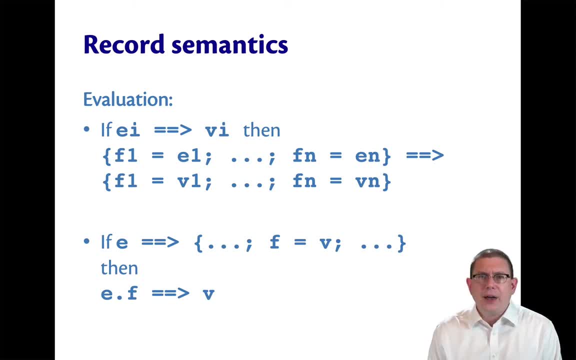 Just evaluate all of the expressions to values. So if you have a bunch of expressions E sub 1 up through E sub n, I'll just say E sub i for all of those. If E sub i evaluates to V sub i for all of them. 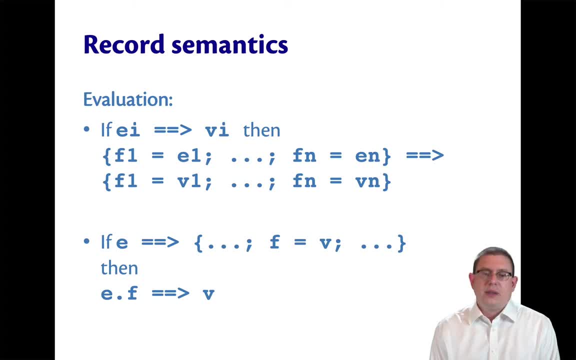 then the record expression with all of those Es evaluates to a record value that just contains values inside of it. And as for field access, if E evaluates to a record value and that record value has a field named F which is bound to a value V, 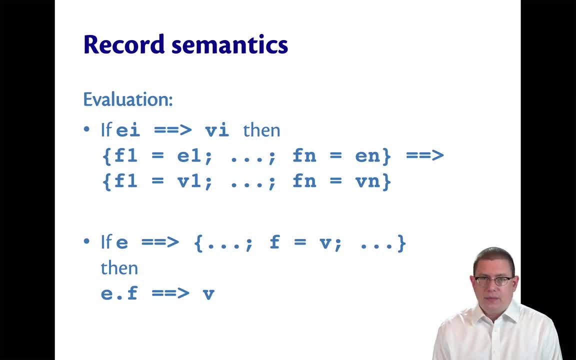 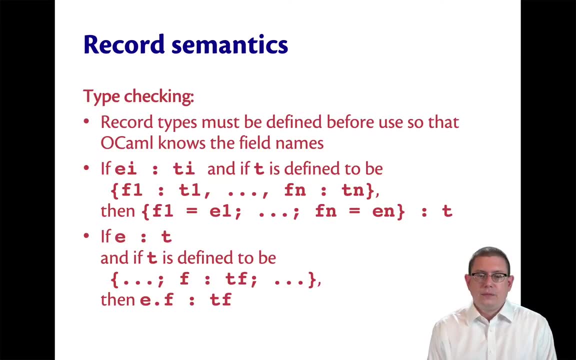 then E dot F evaluates to V. All we're doing is getting the value of that field out of the record For type checking. there's one little quirk here, which is that record types must be defined before you use them. Actually, this is not so surprising. 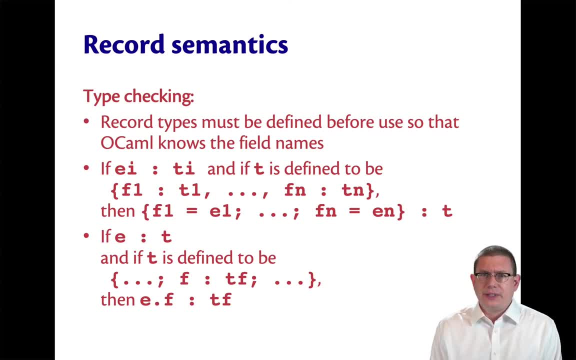 You can't use classes in Java before you define the class. for example, You can't use record types in OCaml before you define the particular record type, And that's so that OCaml knows what the field names are going to be for that record type. 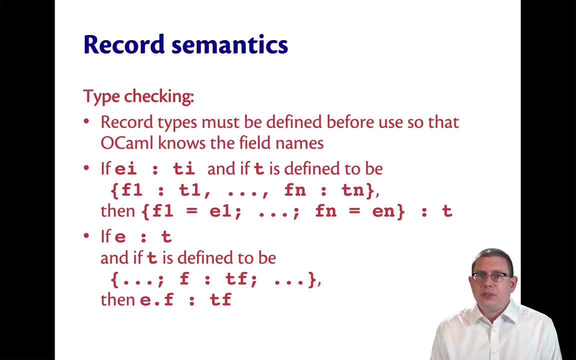 Turns out, it is possible to engineer record types and type inference such that you don't have to define them first, but you don't get as good of type inference for it. Okay, as for type checking rules for records, if you form a record expression, 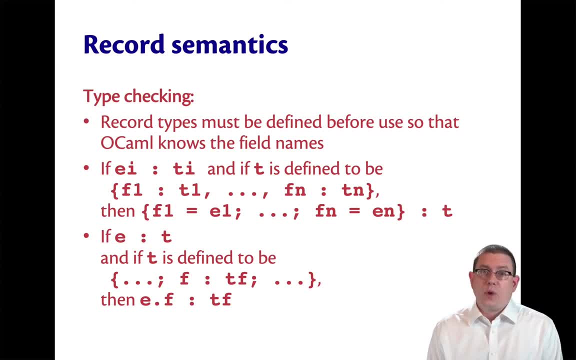 then all of the sub-expressions that are part of it need to have the right type according to the definition of the record type. If you have a field named GPA whose type is float, you can't stick an int into it, And if you go to access a part of a record with the dot notation, 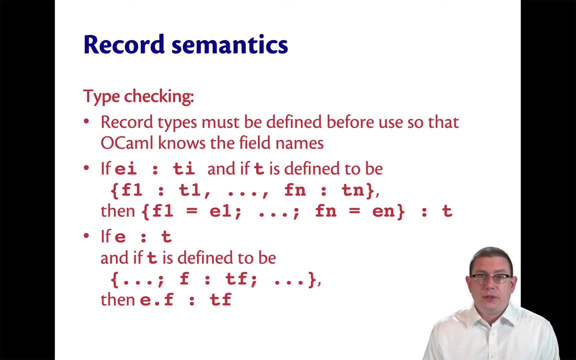 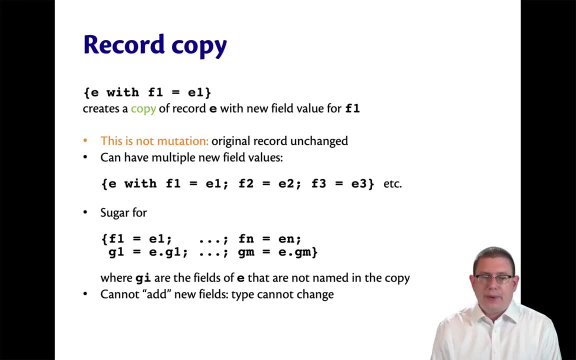 then you get the field of the appropriate type out. One other piece of record syntax that we haven't seen so far is record copy. So if you write curly brace E with F1 equals E1, that creates a copy of record E with a new field value for F1. 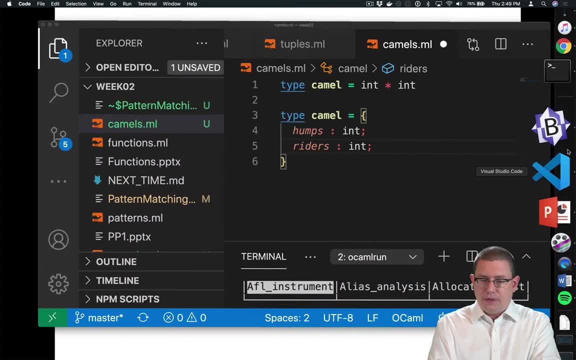 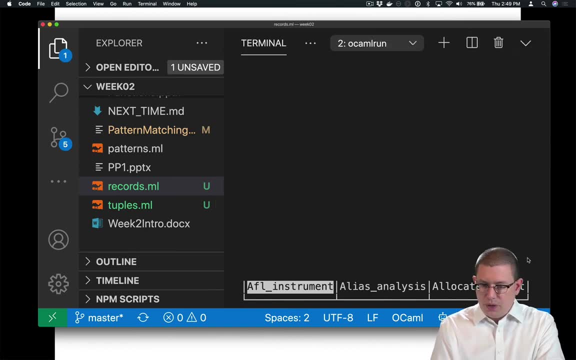 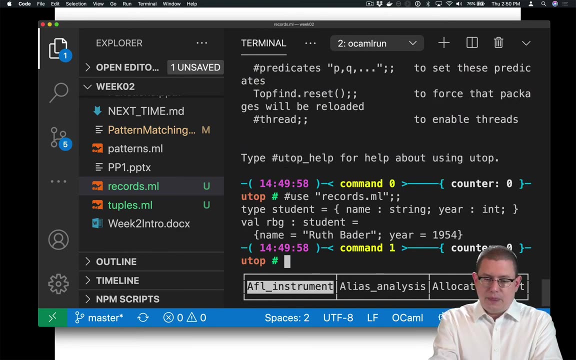 Let's actually try an example of this quickly. Back here we had records and we had RBG. Let's go ahead and load that code into UTOP, Use recordsml. We could create a copy of RBG by writing rbg with. 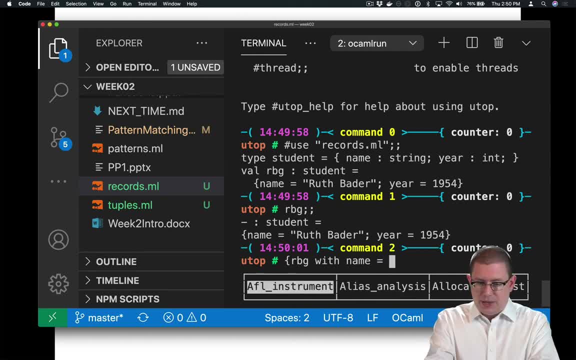 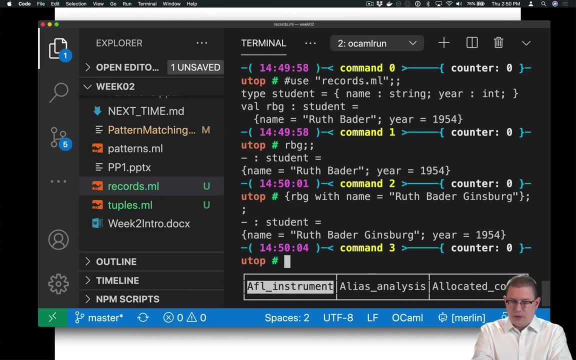 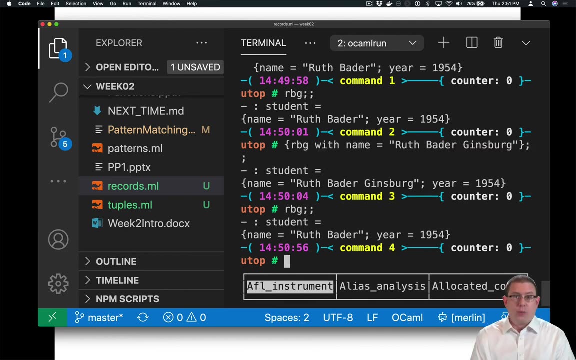 and suppose we wanted to change the name. Name is Ruth Bader Ginsburg. Now we've got a new record in which the name has been changed. Now this didn't go back and change the original record. It's immutable, as always, still just Ruth Bader. 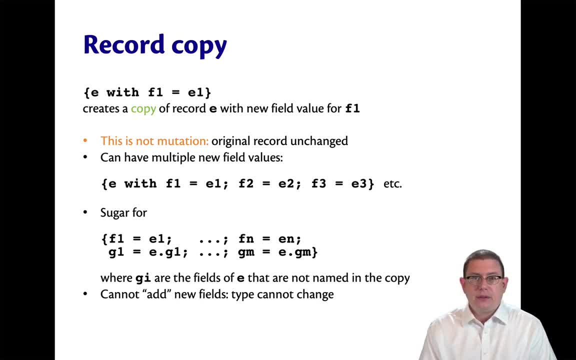 So record copy is not mutation. It leaves the original record unchanged. You can also replace many values if you want at the same time inside of the record by just chaining them on with semicolon. field name equals some expression In reality. record copy is just another example of syntactic sugar, though. 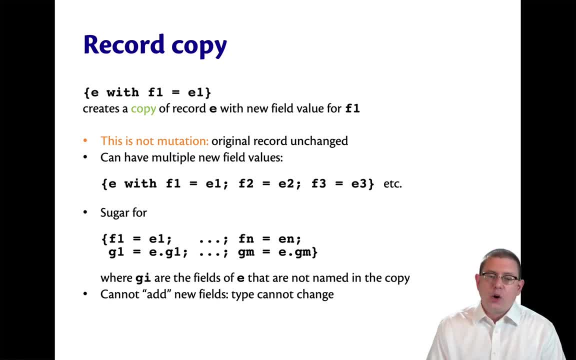 It's really sugar for just rewriting the entire record with all the field names, using all of those field names in the with clause And then all of the field names that you didn't happen to mention in the with clause from the original record. But it's much more convenient to be able to use the record copy syntax.